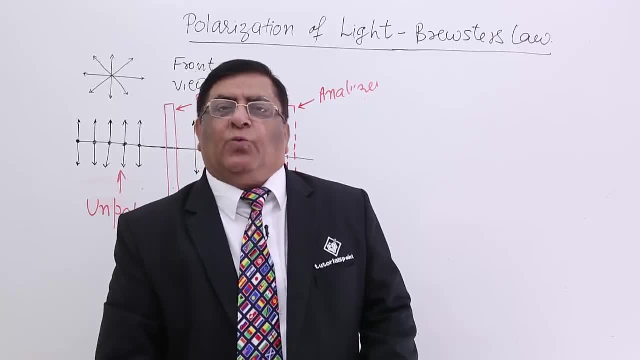 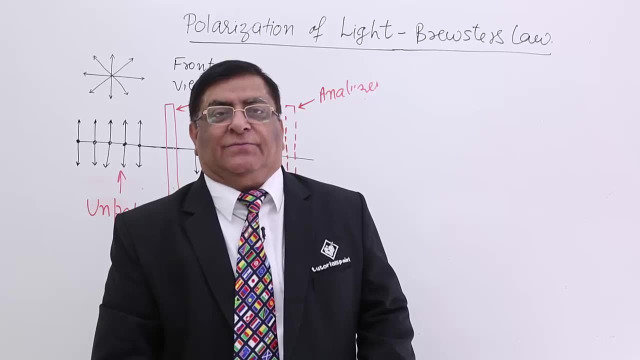 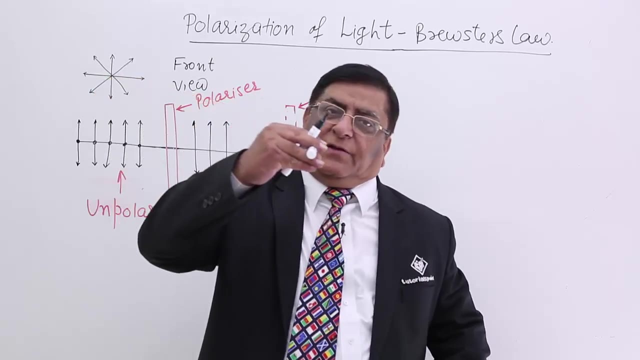 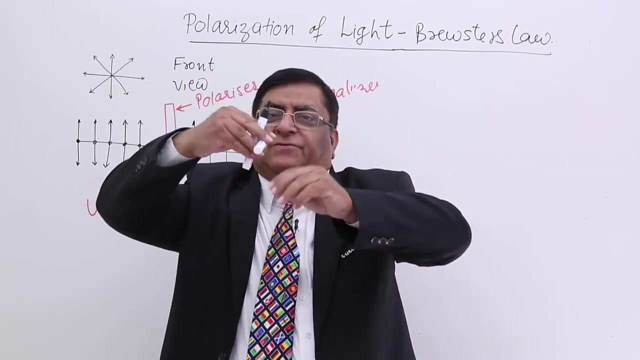 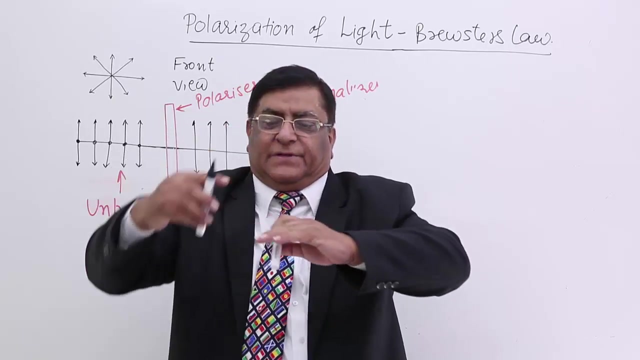 There are many methods of polarization and one of the method is polarization by reflection. How polarization by reflection? It is very interesting. This is the light which is coming towards a surface. Light coming towards a surface. There are certain vibrations in this direction which are perpendicular to the surface, perpendicular plane of the surface. 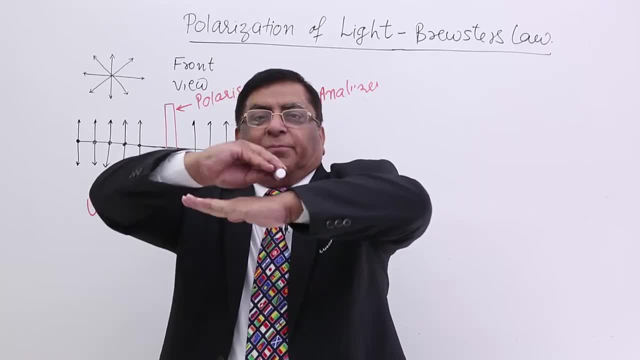 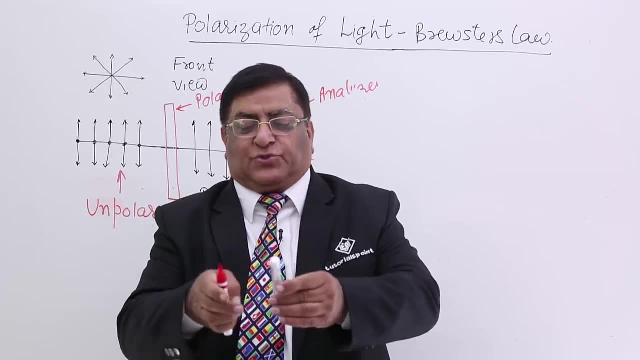 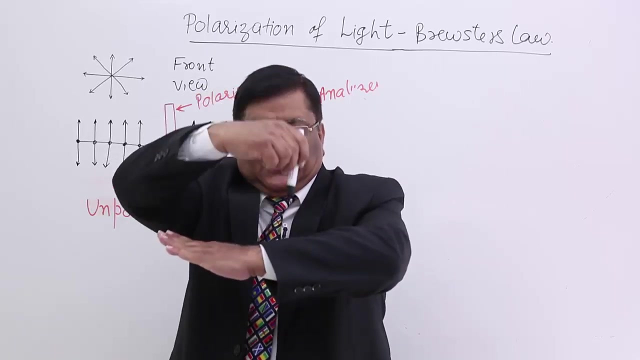 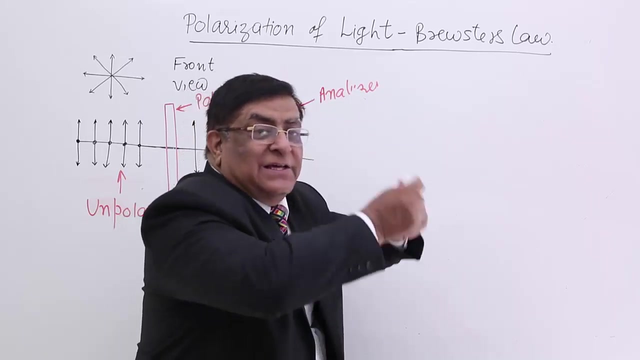 There are certain vibrations which are in the plane parallel to this. Now both of them come and strike this. There is a certain action. This comes and strike like this. What will happen? Just as if somebody is, If somebody is digging the earth, this, If it strikes like this, there is a chance. 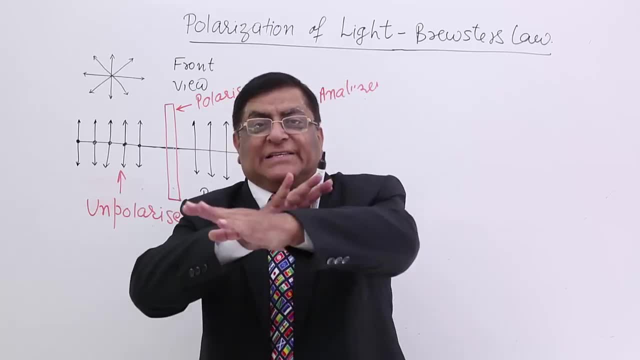 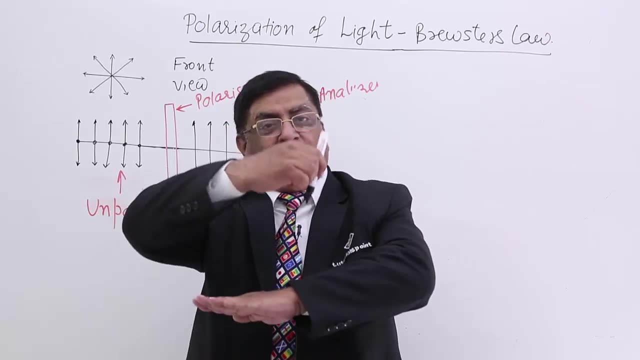 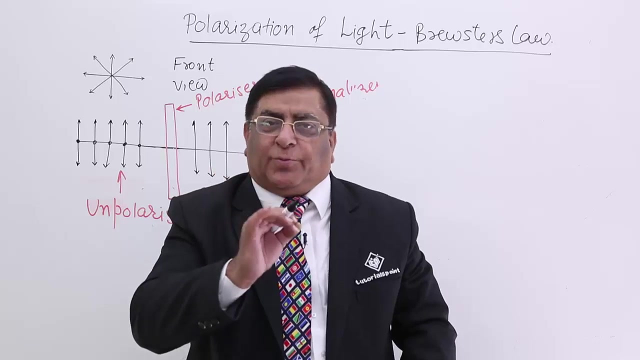 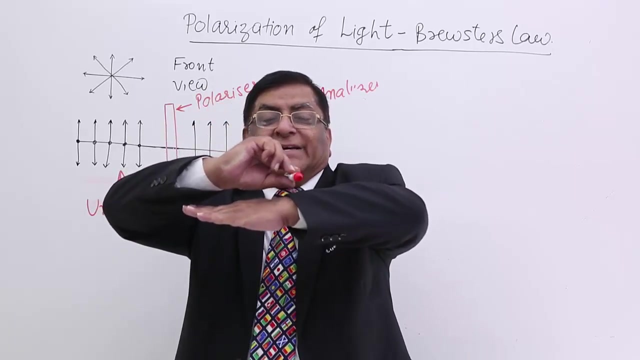 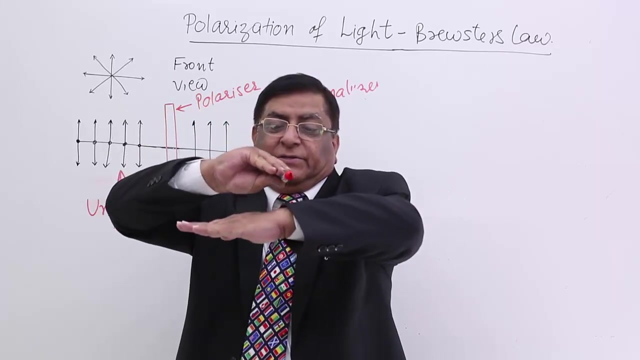 that this will be absorbed. If this is a transparent surface, it will enter. If this is not a transparent surface, it will be absorbed. The chances are that it will get destroyed, either by absorption or by transmission. What happens to this? It does not strike it by the corner, But it simply goes like this. And when this strikes, 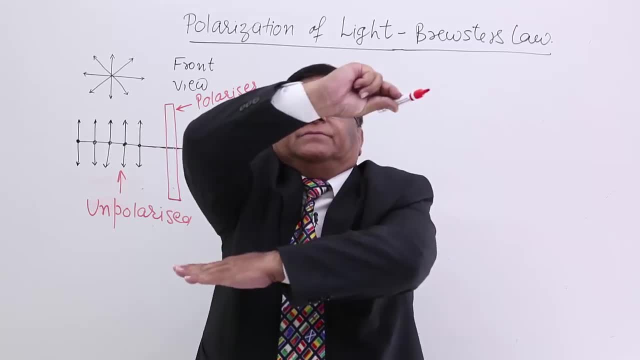 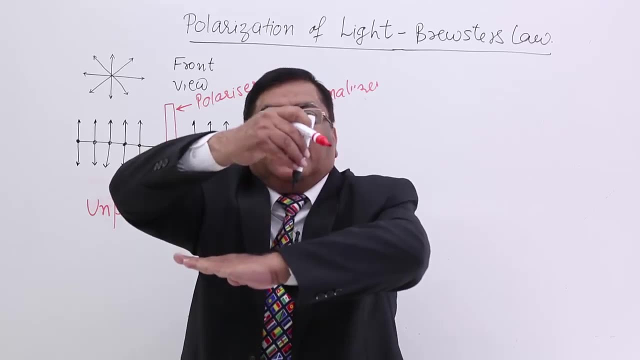 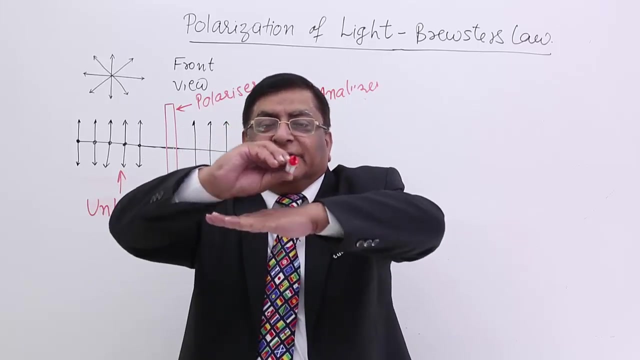 this way, it just jump, reflect. You can imagine If this strike this way, it will strike, get absorbed or enter. This is not striking by this direction. This is a direct energy that is coming here. That would be a straight energy. You can explain this. 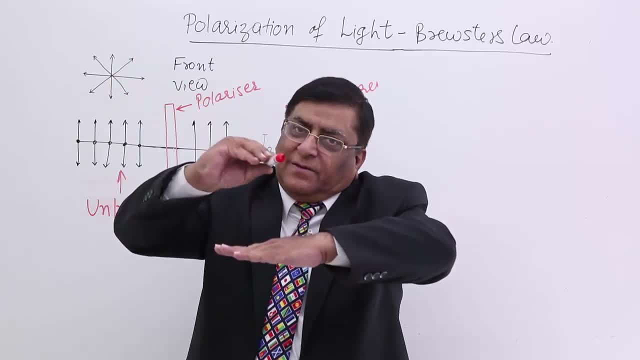 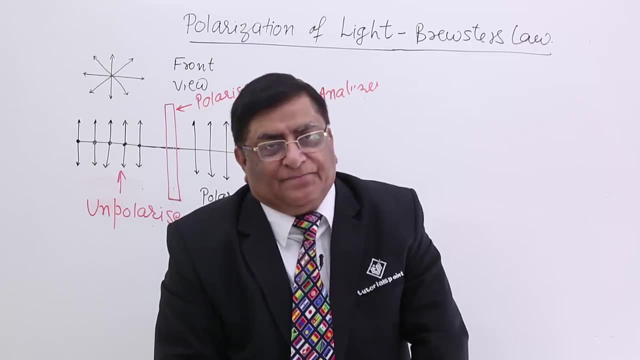 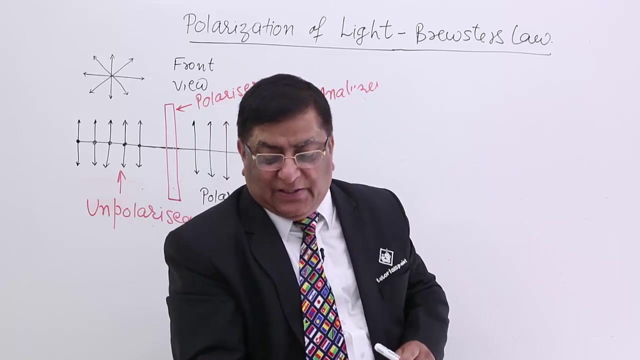 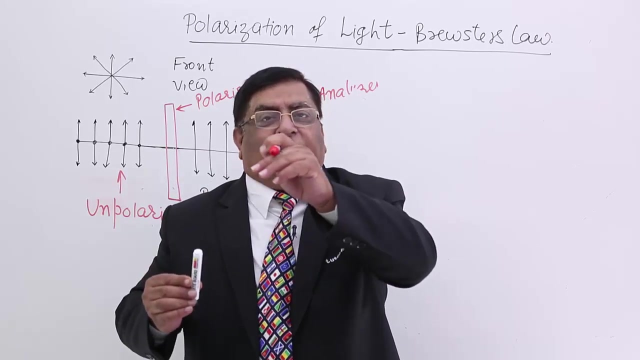 striking that way. this is just coming this way and this is the speed. when this strikes, it gets jump and gets reflected. So in the reflected light we see lot of it and we see very less of this. So one type of vibrations are in majority and other type of vibrations are in minority. 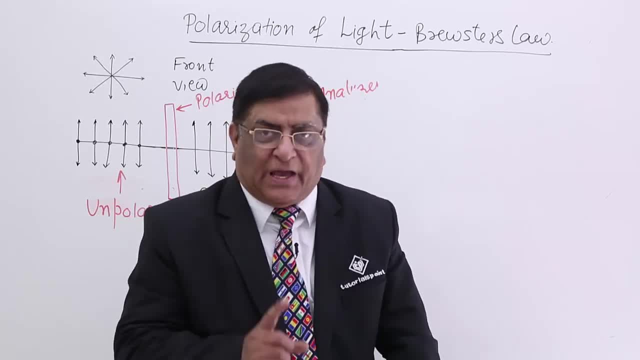 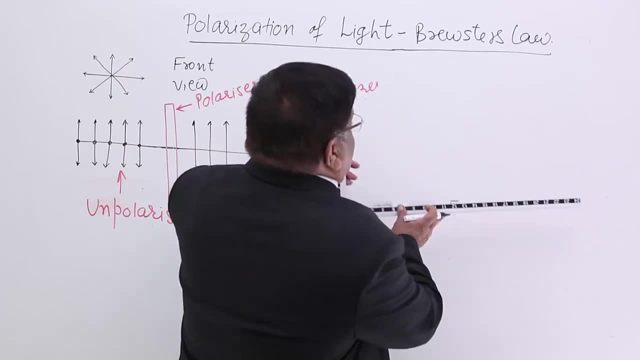 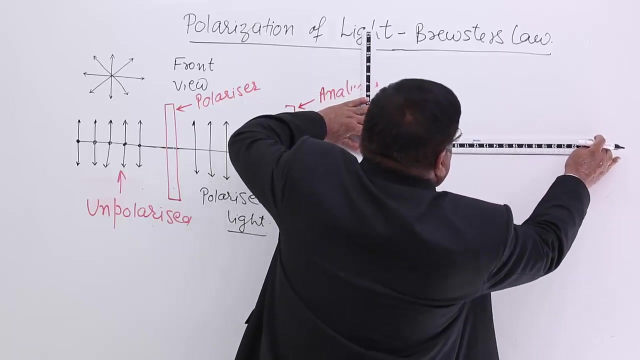 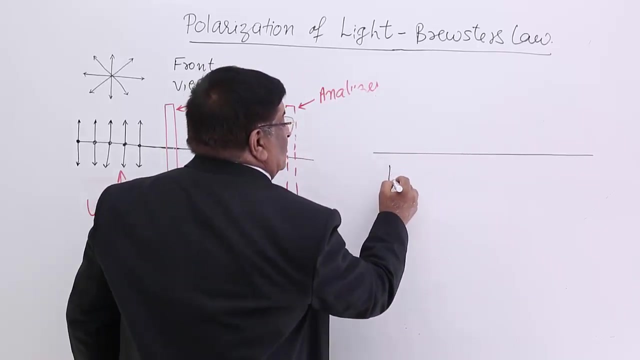 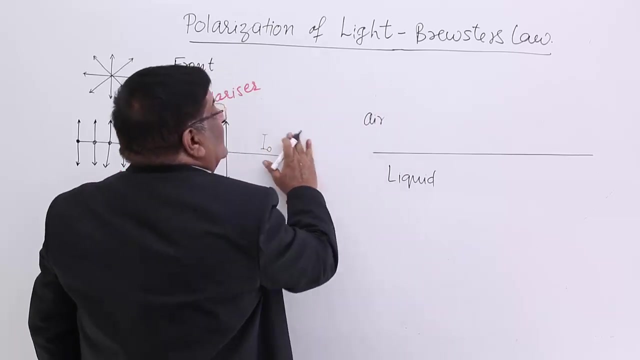 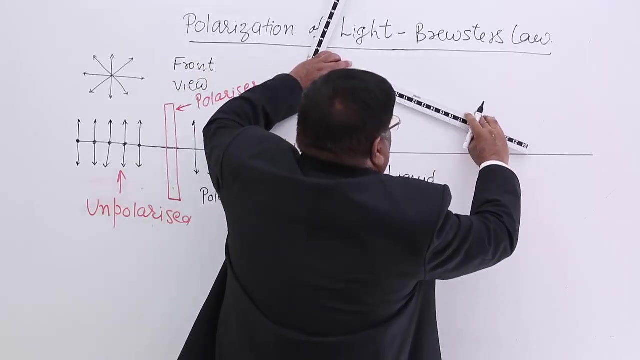 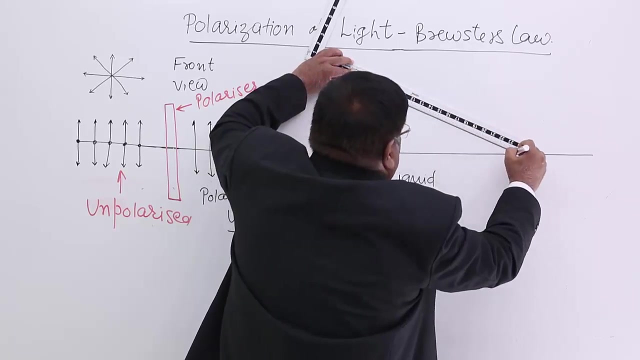 and that is polarized light. So I will draw it. we have a surface, let us say, and this is the interface between a transparent medium, say liquid, and this is air. In the air, a light is coming which is not polarized. If it is not polarized, then this is the direction of approach and the vibrations I will exhibit. 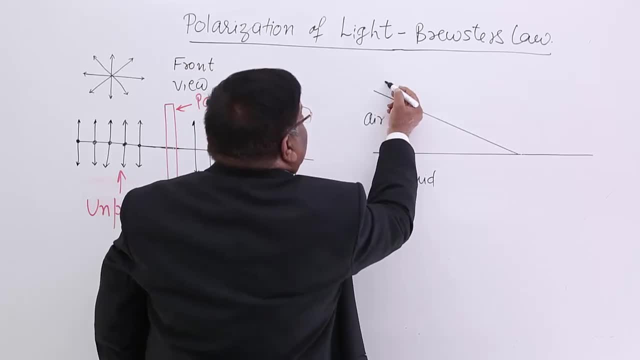 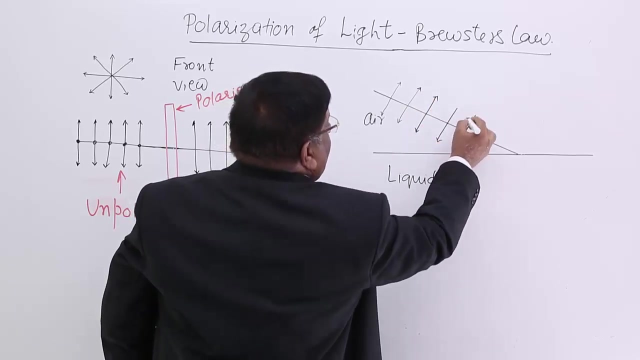 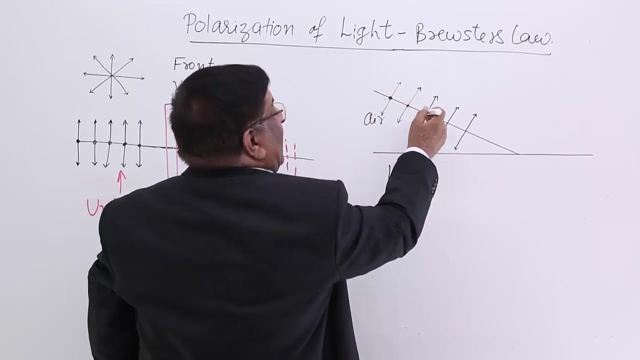 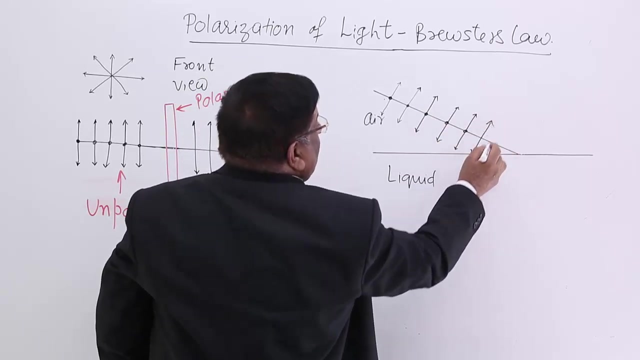 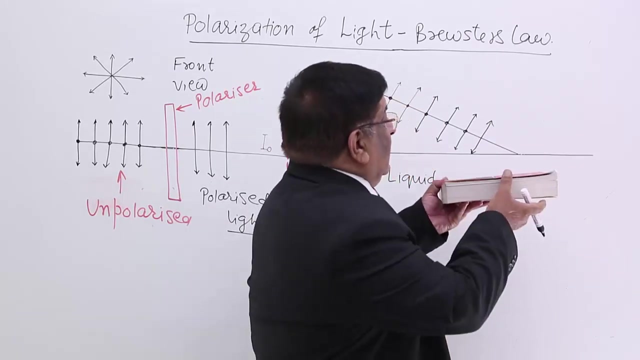 in two directions. One is this, which is perpendicular. this one, This one And other vibrations are in this direction. What is this direction? This is the direction of this pen, this. So, if this is the surface, If this is the surface, 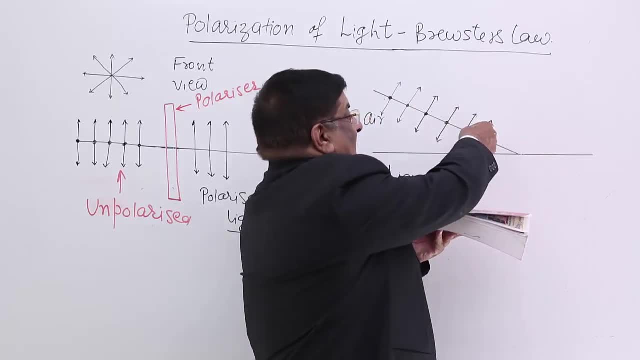 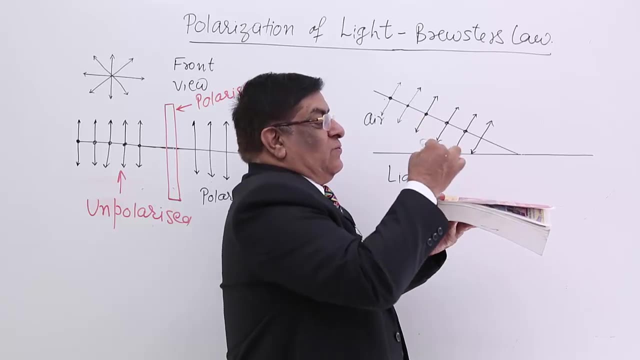 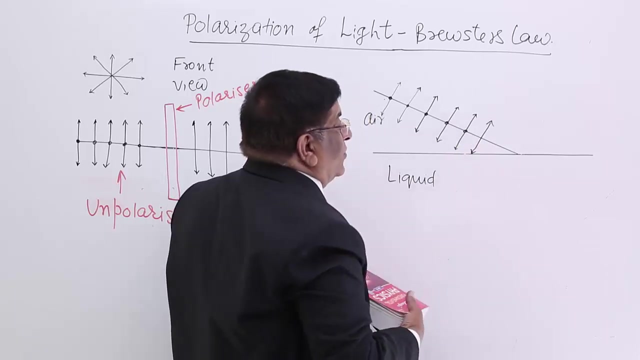 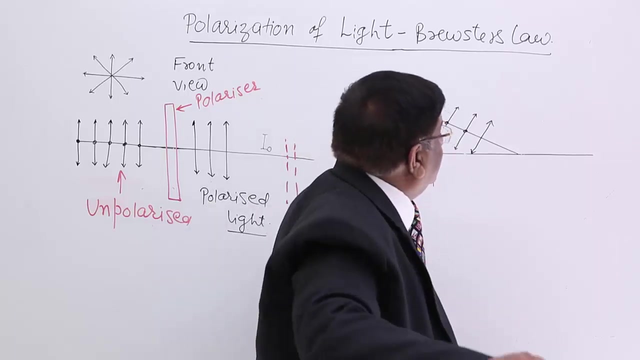 Then the light which is coming from here has certain vibrations this way and certain vibrations this way. This, when strike here jumps. Which one? This one jumps, and the rule is angle of incident is equal to angle of reflection, So I get the reflection in this direction. Okay question: What is the angle of? How much is angle of? This is a revolution. What is the angle of direction? Let me add here P in it. here it is equal in ecb and I can say it here: it is equal in ecb. and 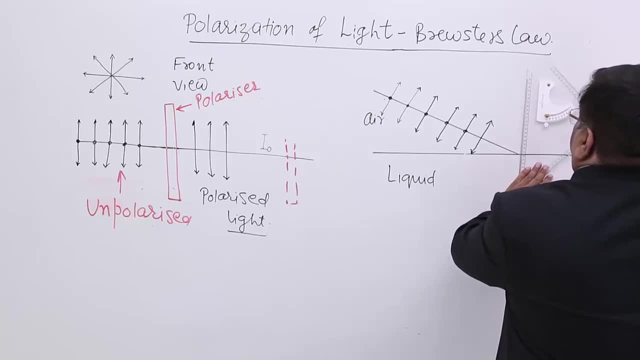 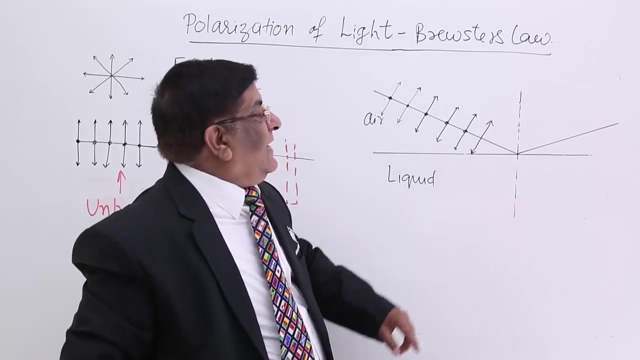 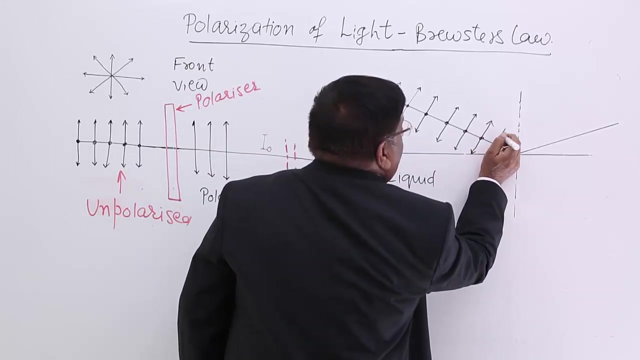 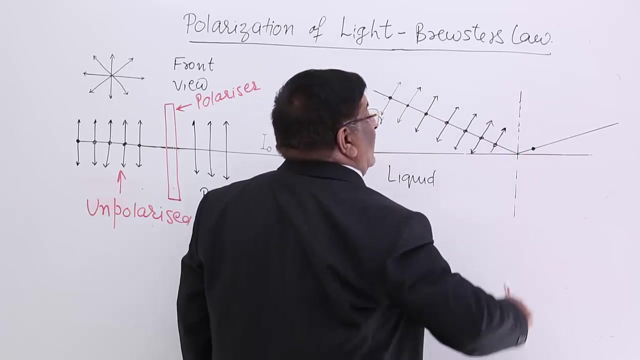 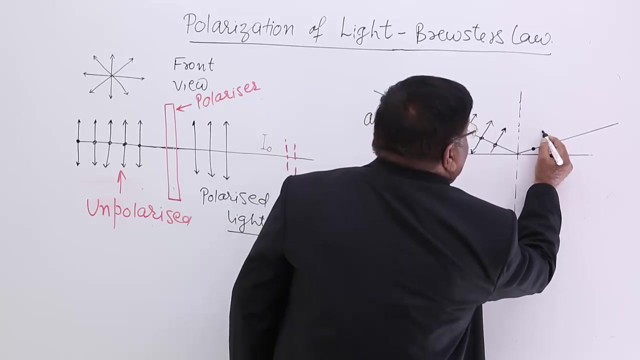 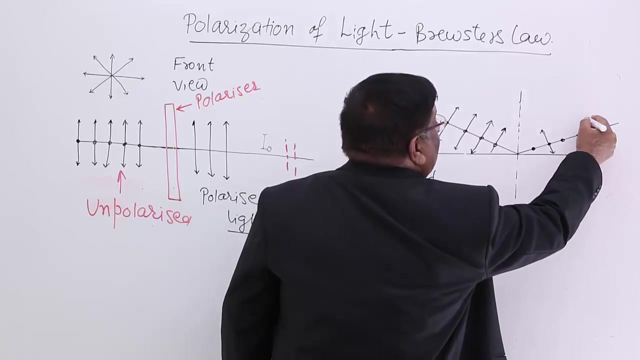 Let us draw a normal here, and this is the angle. I is equal to R. but in this reflected light, what do we see? Here we see this vibration and that vibration gone. Here we see this vibration and that vibration, both Here- this vibration, this vibration- and here again. 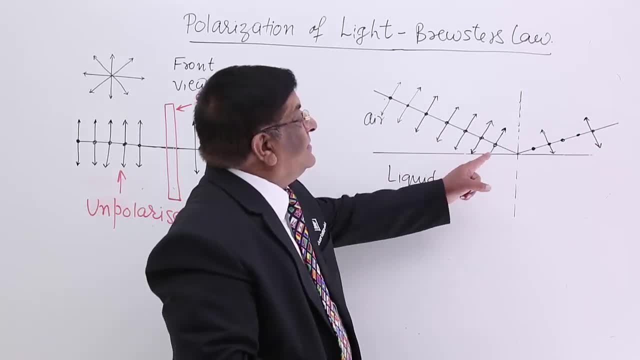 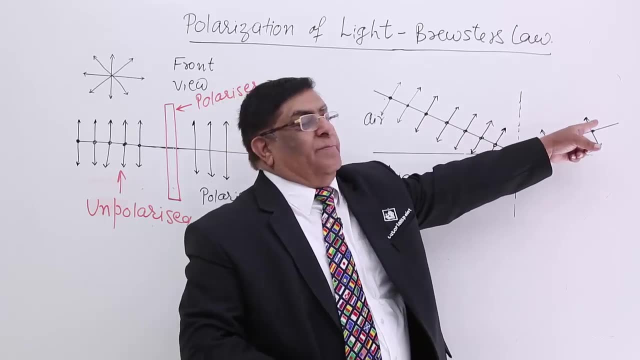 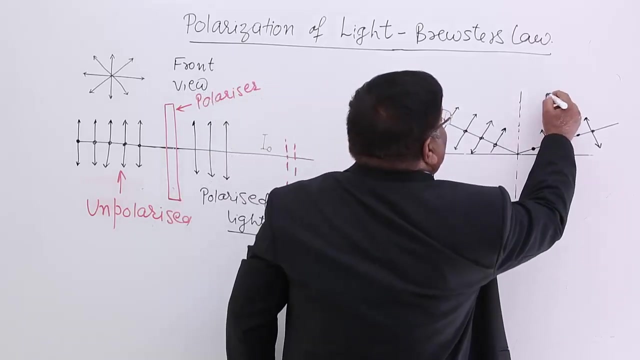 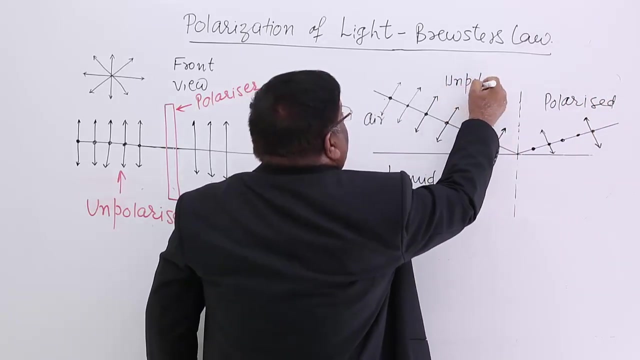 So some of these vibrations may come, and most of these vibrations do not absorb, and they come here. So what is the light? This light? what we get is polarized light. This is unpolarized. This is unpolarized light. This is polarized light. 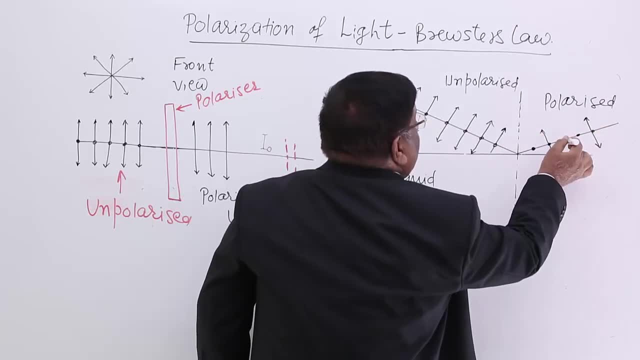 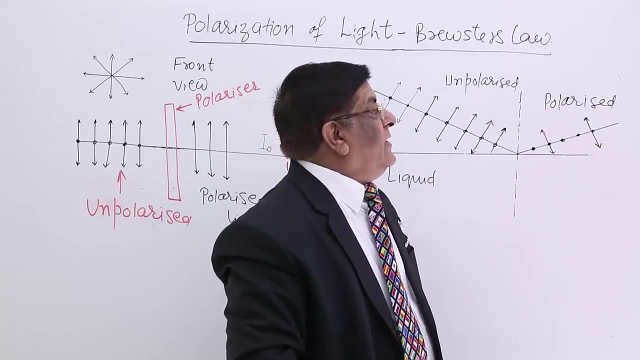 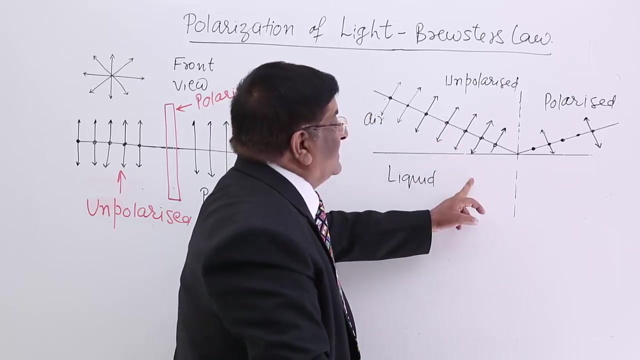 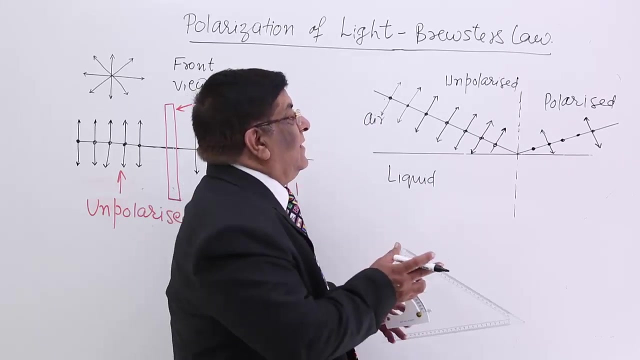 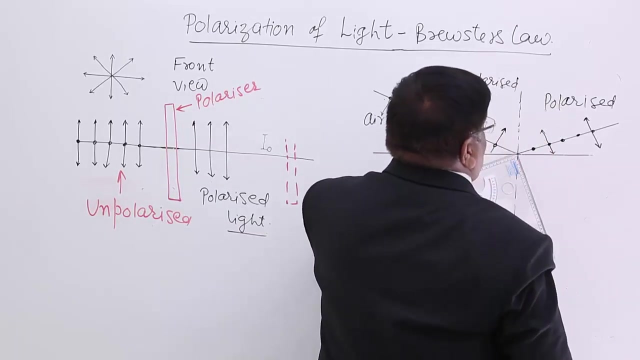 Because it has got the vibrations more in one direction, less in the vertical direction. Some part of this light is also some part of this- is refracted. That refracted light enters the medium liquid and that makes a very unique thing. It is refracted in this. 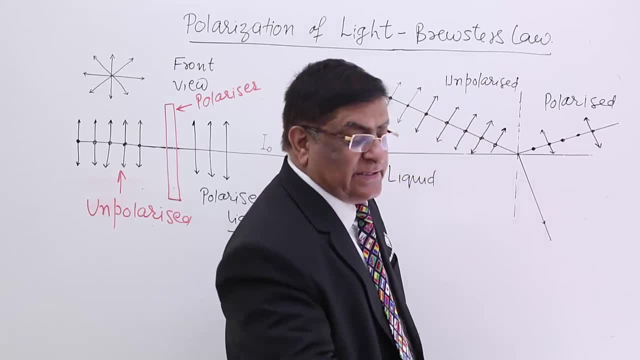 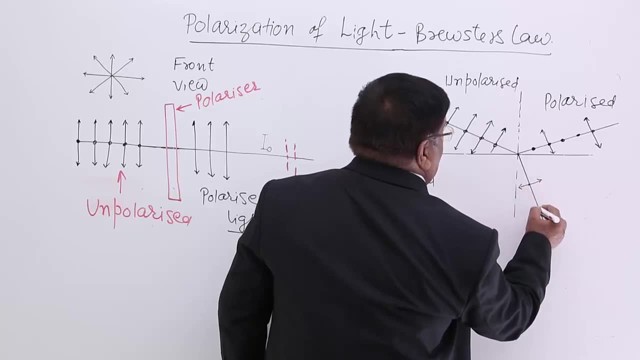 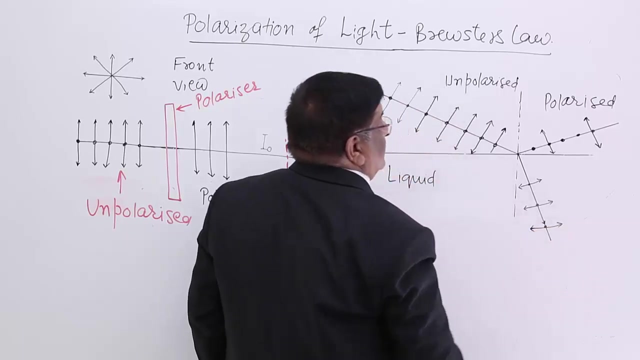 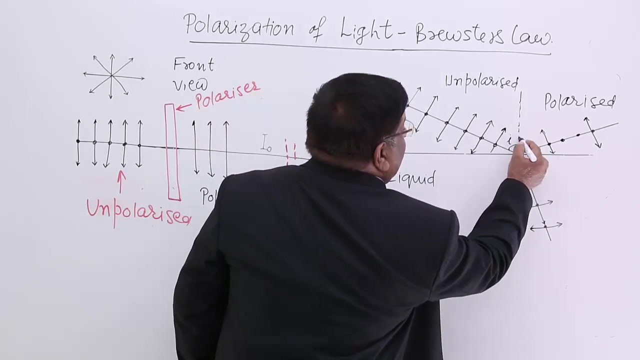 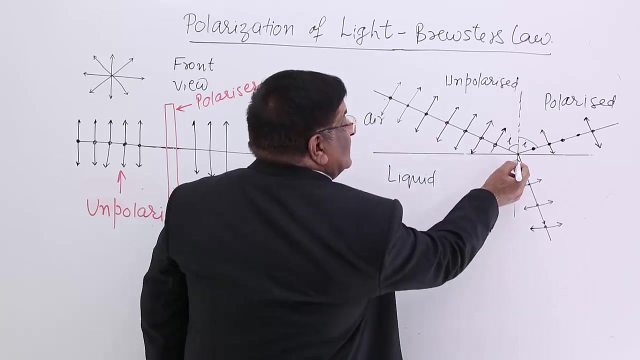 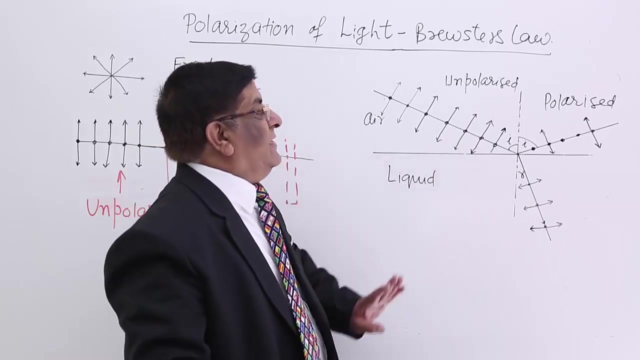 direction, but this is not necessarily polarized, So it has got vibrations in both directions this way. Now, this is certain angle I and accordingly this is angle of refraction, which is also equal to I. This is angle of refraction R, so that mu is equal to sin I upon sin R. This is happening. 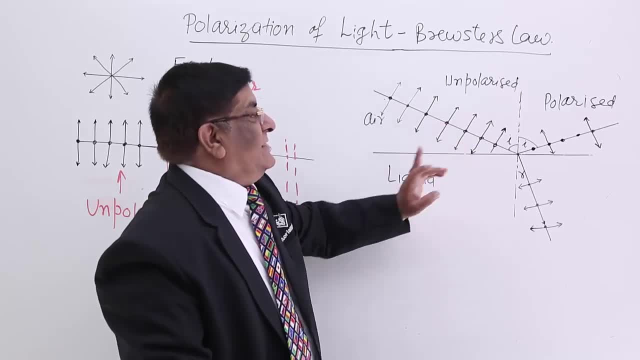 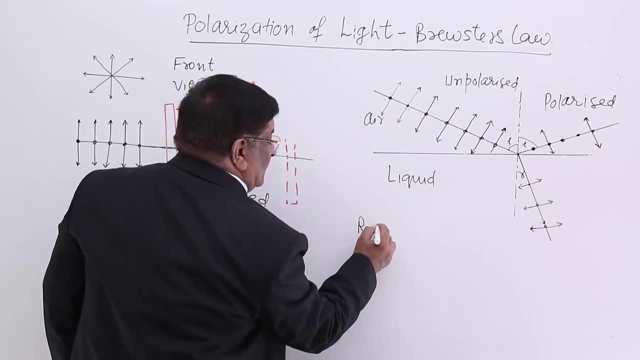 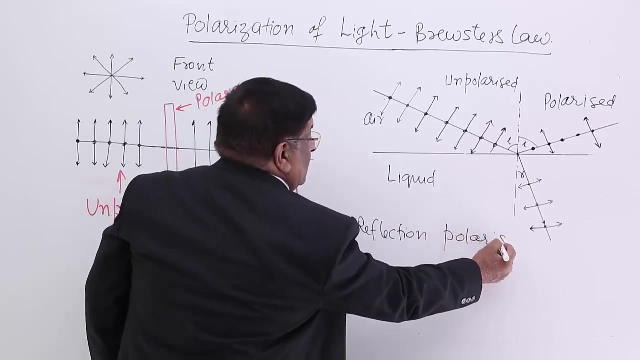 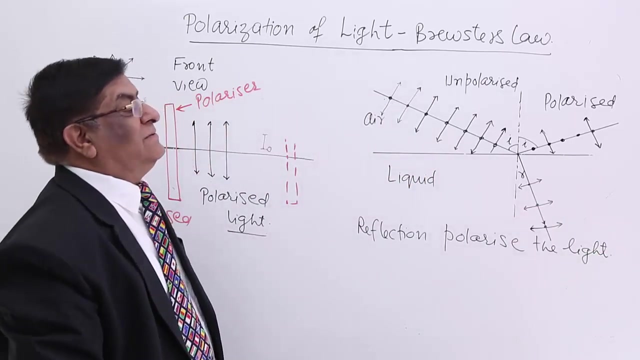 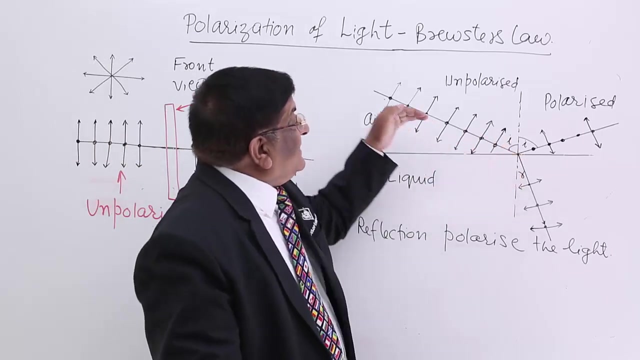 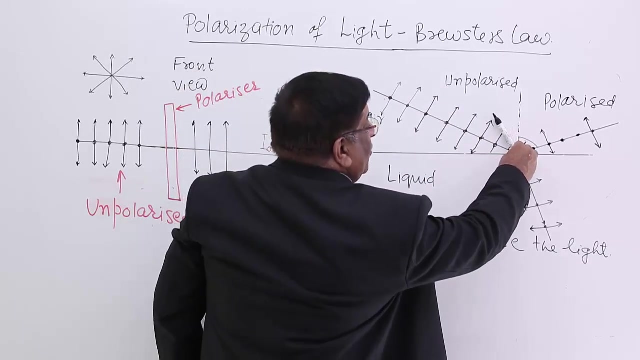 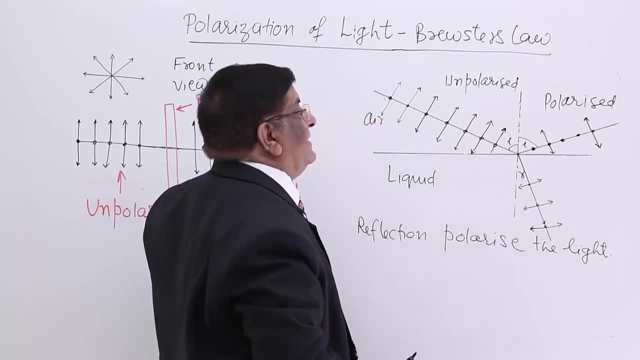 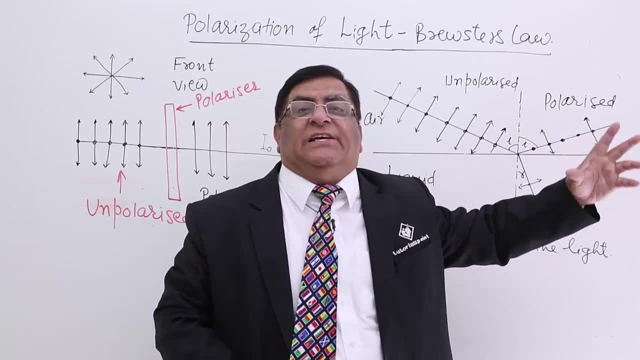 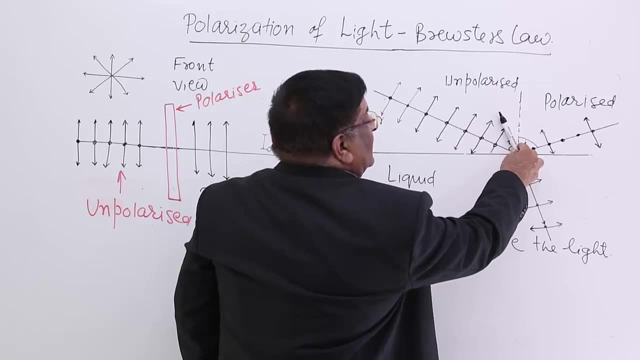 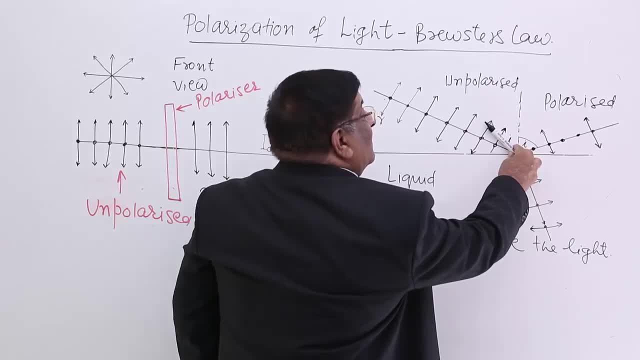 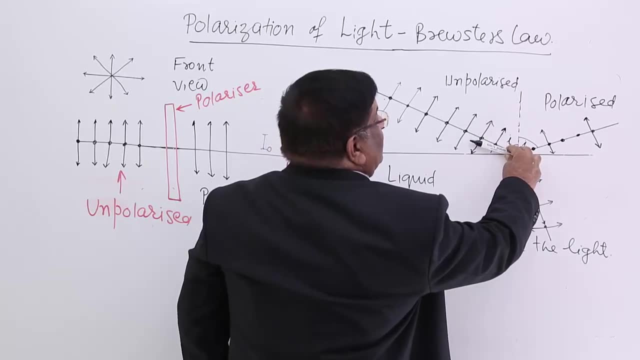 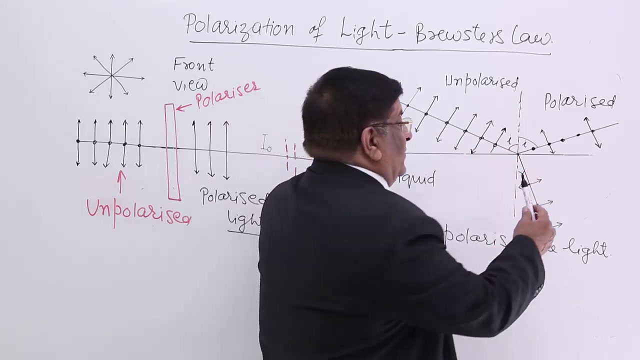 increase. here the polarization become 100 percent again. polarization 80 percent, 70 percent, 60 percent, 20 percent. So the polarization percentage: here you see: 1,, 2,, 3,, 4,, 5 and 2, how much polarization. 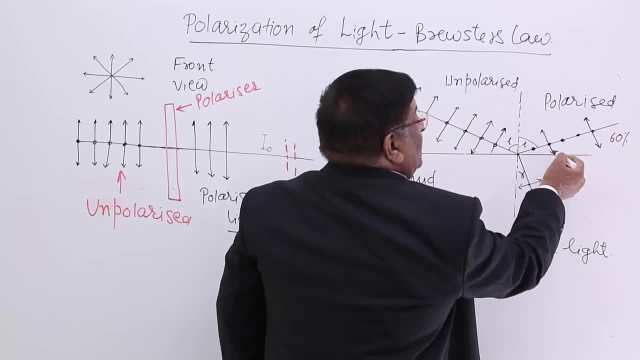 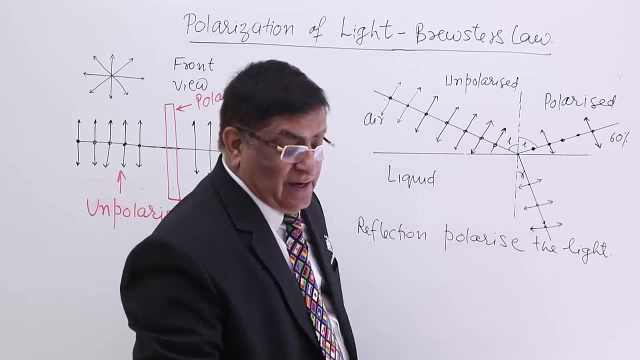 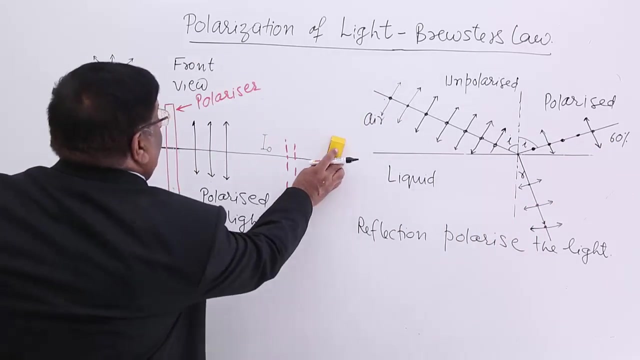 is there: 60 percent. 2 are not polarized, 3 are polarized: 60 percent polarization. So when we change this angle, I we find that the percentage of polarization keeps on changing. So that I will write here: 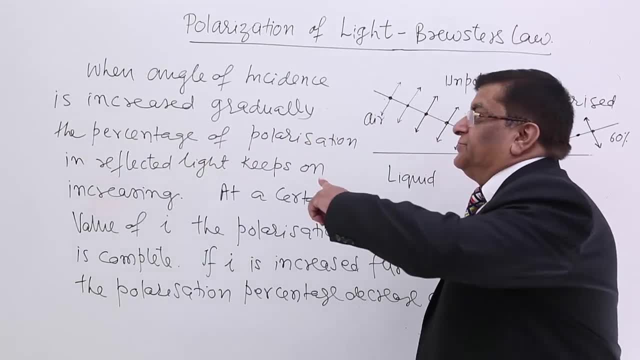 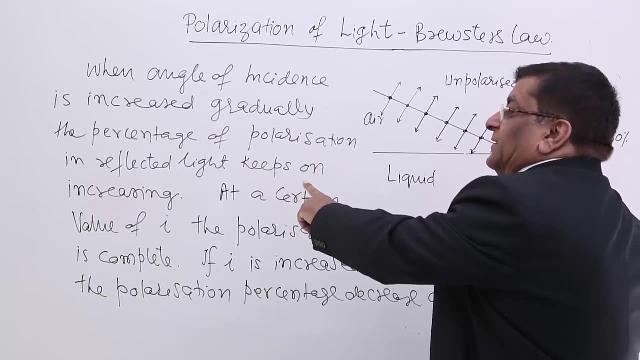 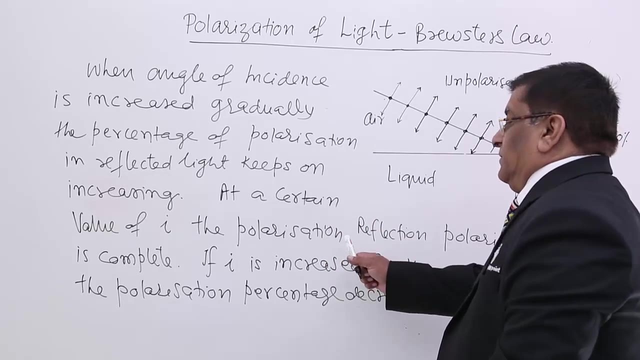 The sequence: See. I have explained the situation. When angle of incidence is increased gradually, the percentage of polarization in reflected light keeps on increasing. At a certain value of I, the polarization, the polarization is complete. If I is increased further, the polarization percentage decrease again. 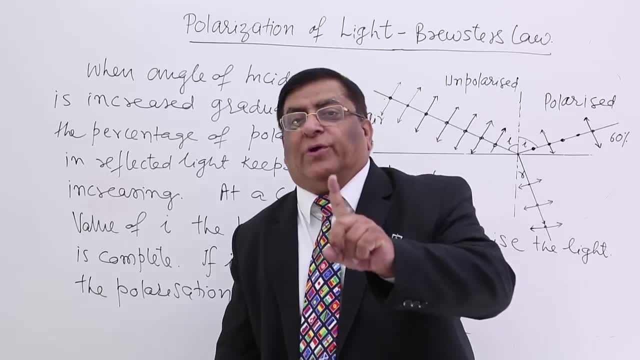 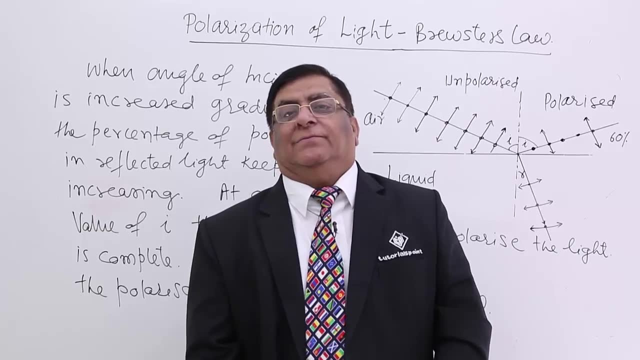 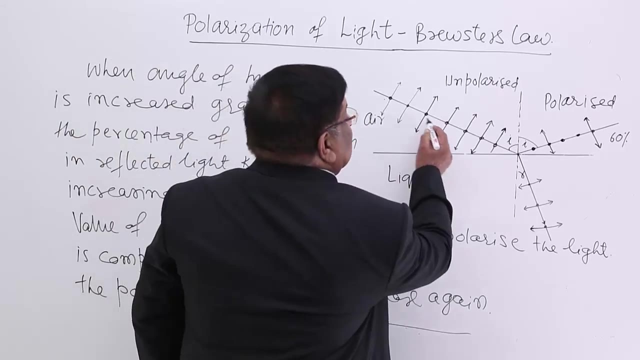 That means there is only 1.. There is only 1 value of I for which polarization is complete, And that angle I is known as polarization angle or Brewster's angle. So that will be somewhere. Let us suppose this is that angle. 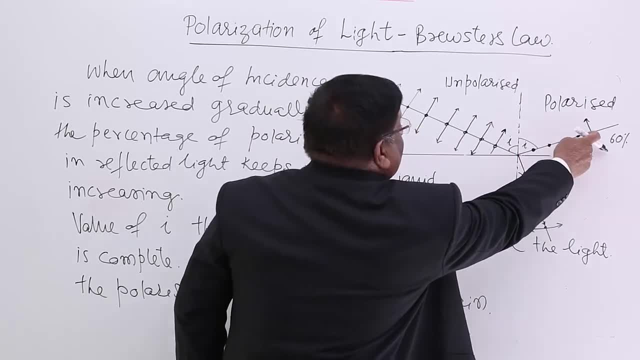 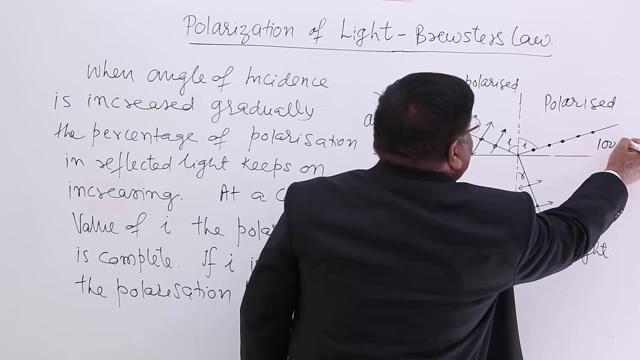 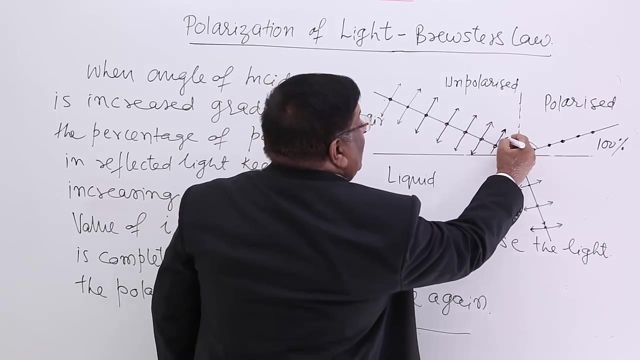 If this is that angle, then what will happen? This polarization will be 100 percent, 100 percent. So this is 100 percent, This is 100 percent, This is 100 percent. So if this is 100 percent, then this angle is angle of polarization, or Brewster's angle. 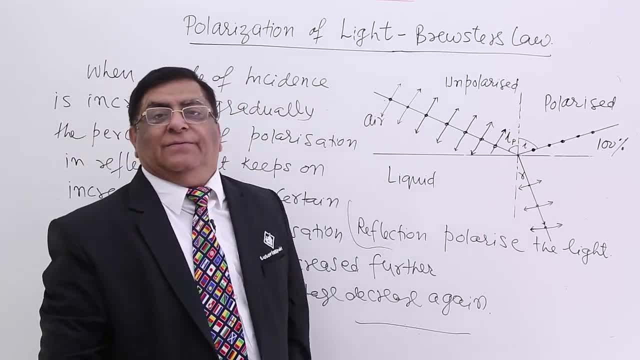 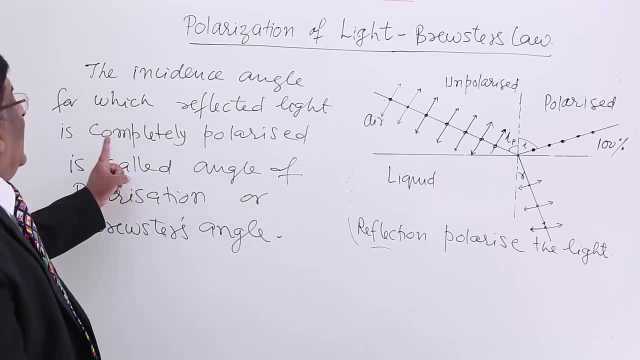 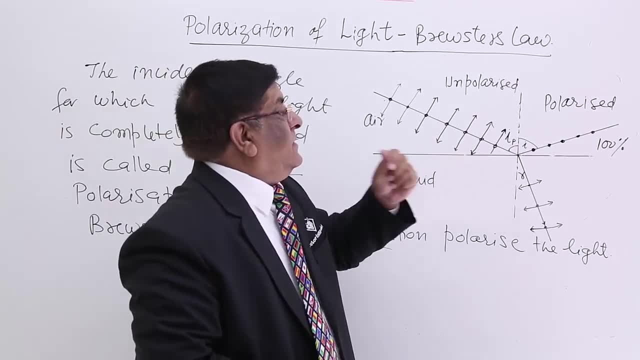 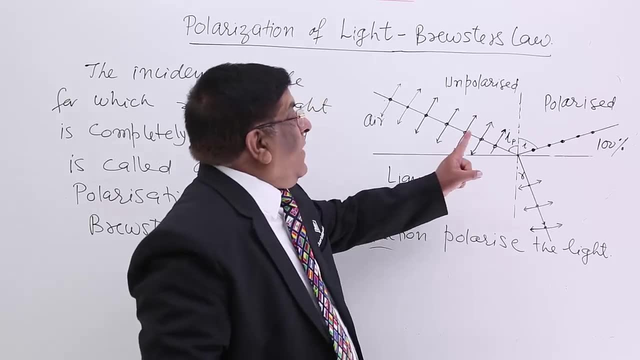 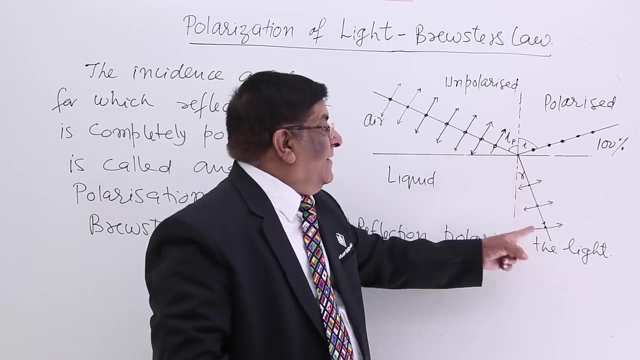 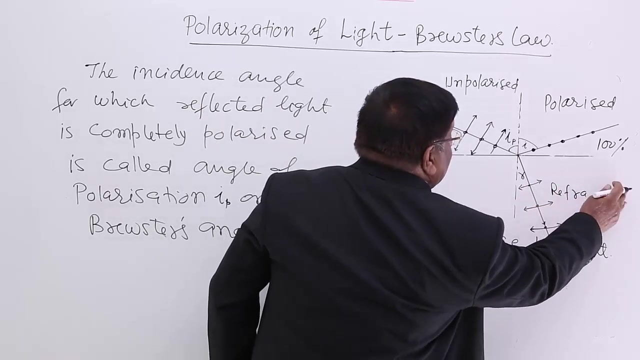 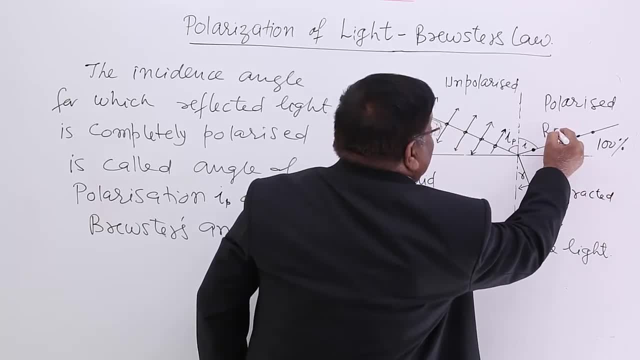 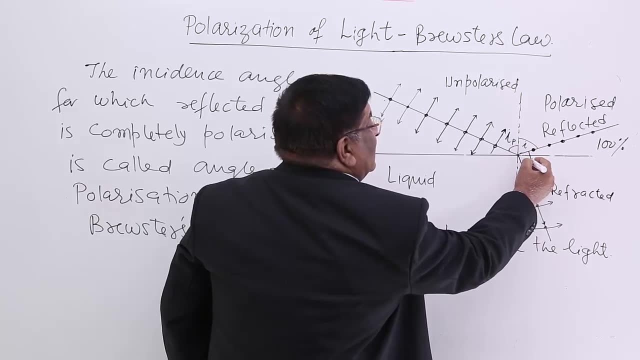 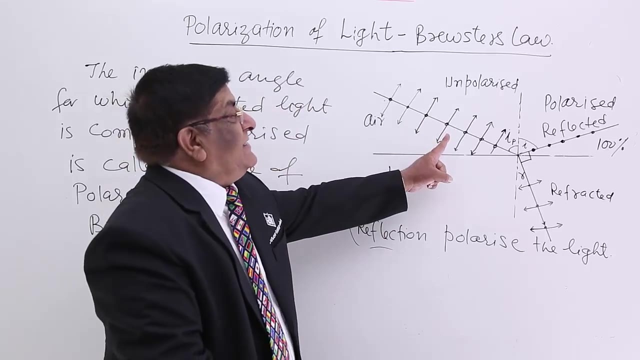 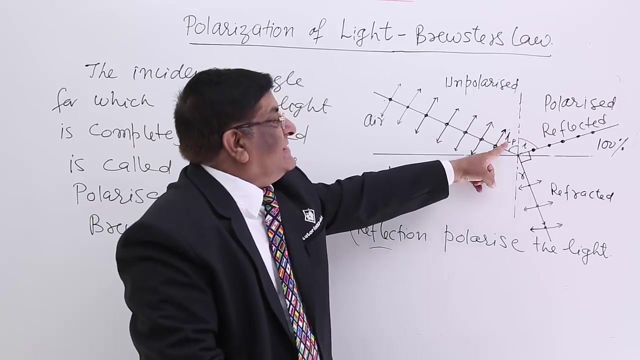 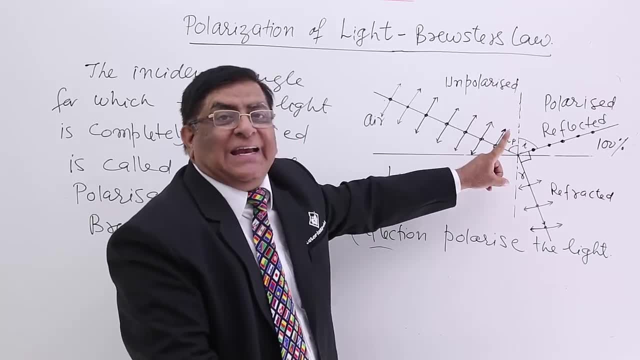 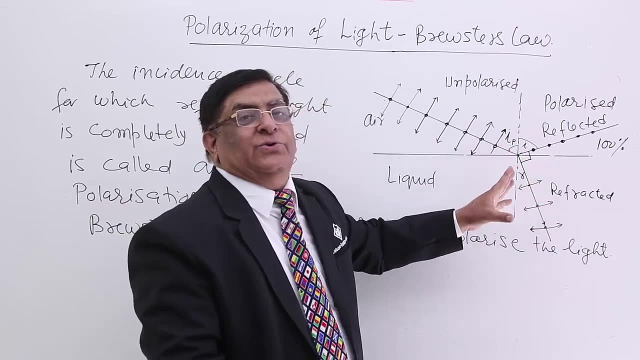 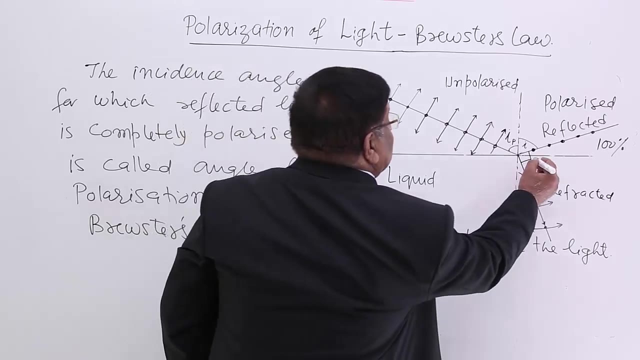 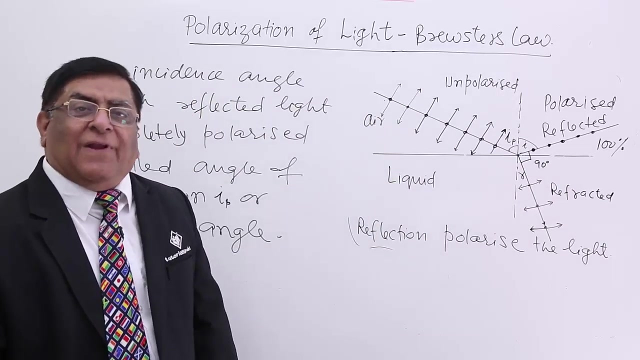 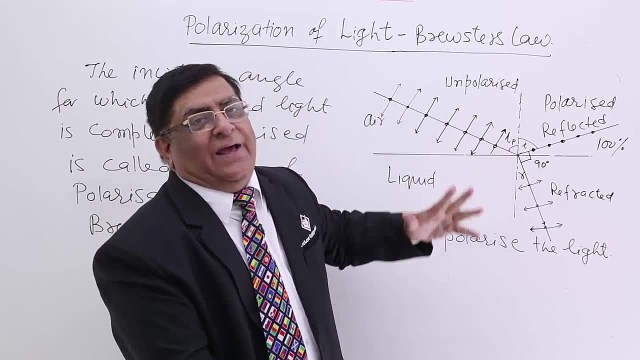 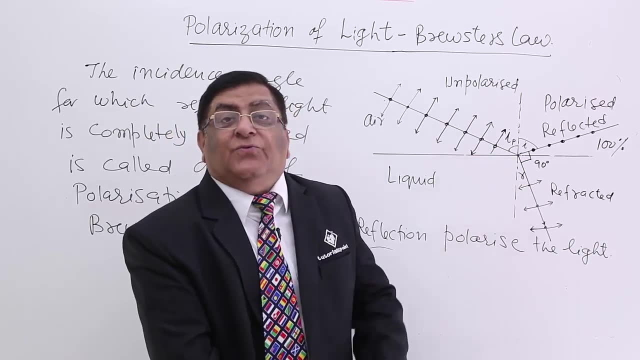 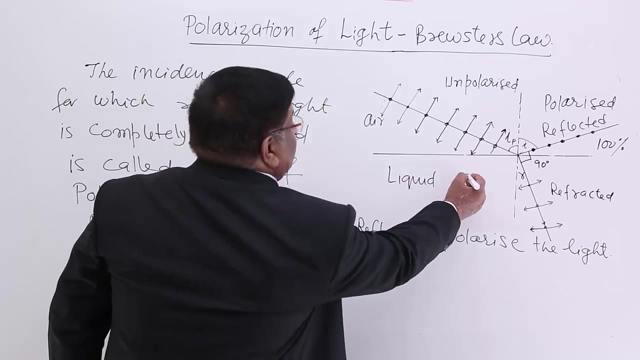 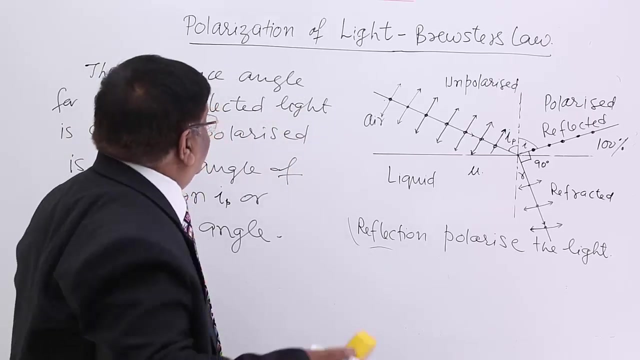 This happens when this angle is Brewster's angle. Now, when this angle is Brewster's angle and this angle has become 90,, we found another equation for refractive index, Mu of this medium. Now, Mu for this medium is sin i upon sin r. 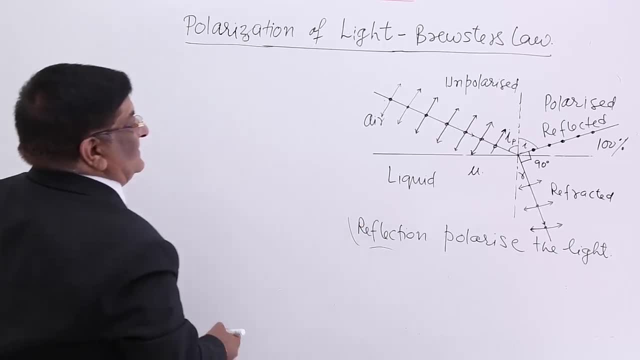 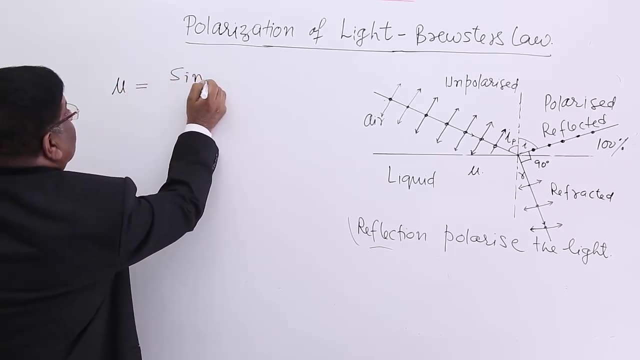 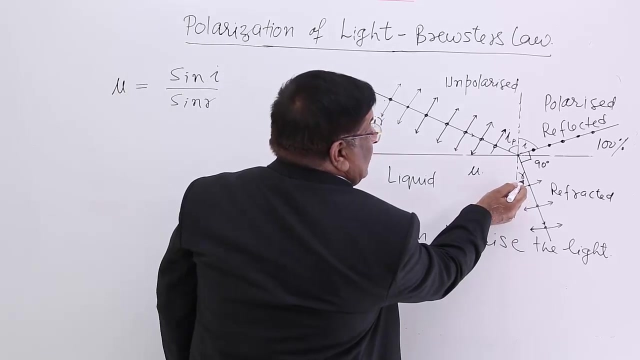 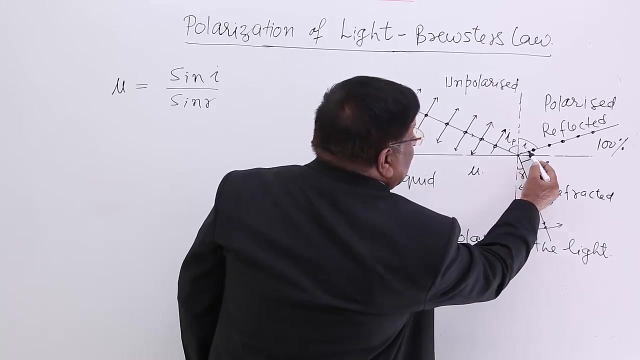 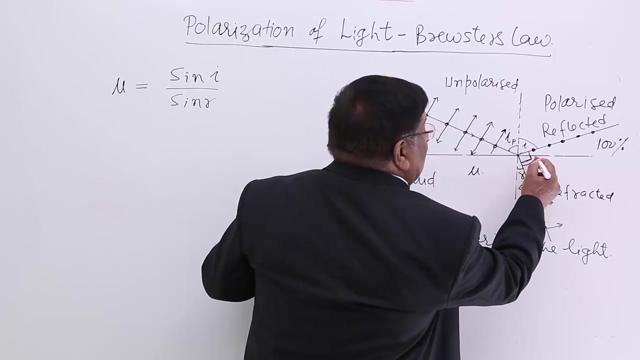 Now we will see the relation with refractive index. Mu. Mu is integral of Re, equal to sin i upon sin r. This is r. Now, if this is r, this angle is 90.. See the angle sequence. I am asking you: How much is this angle? Answer: 90 minus r, If this is 90 minus. 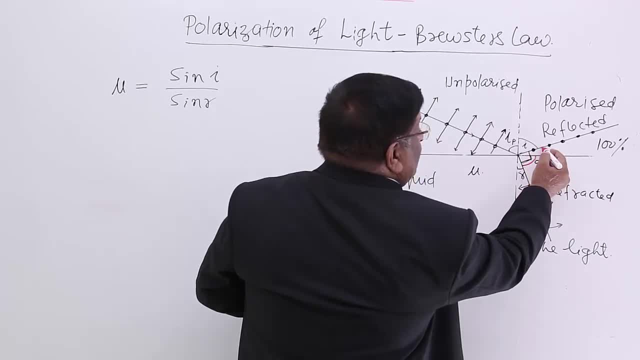 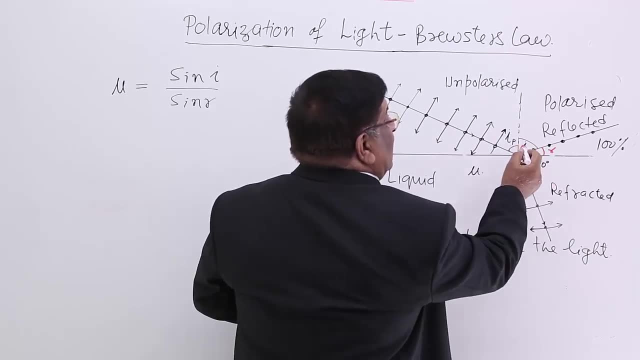 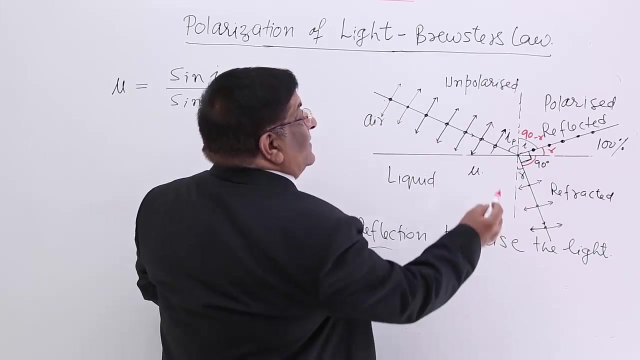 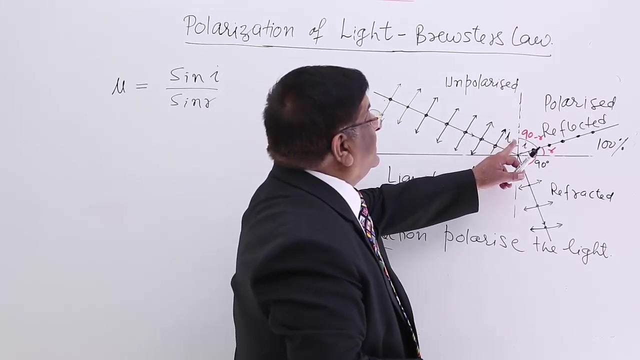 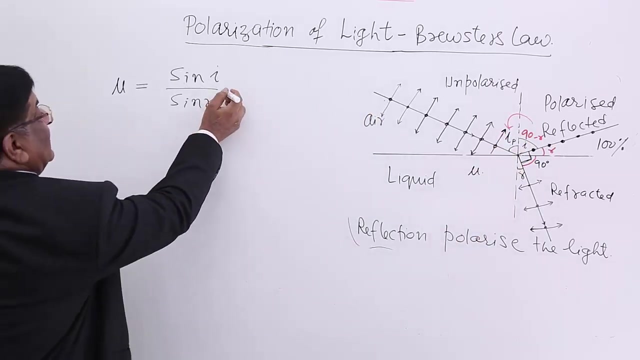 r and this angle is 90, how much is this angle r? So this angle is r. If this angle is r, then how much is this angle? This is 90 minus r And this is equal to i. i, So i is what? 90 minus r. This is also 90 minus r. So here I can write it: sin 90. 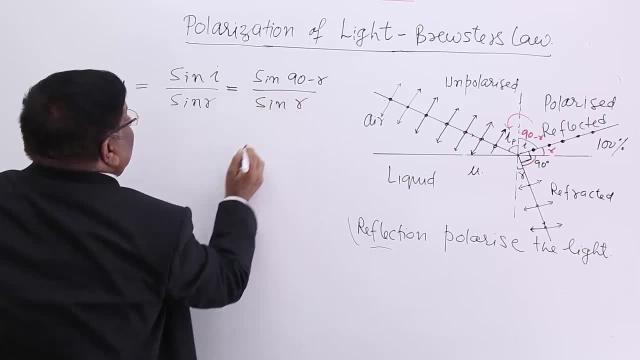 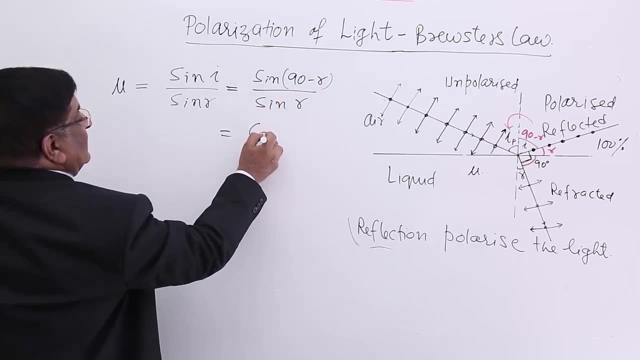 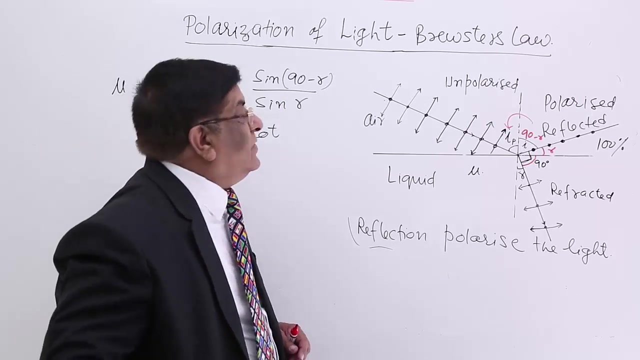 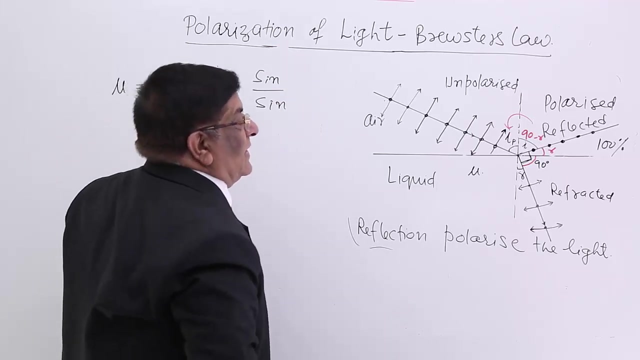 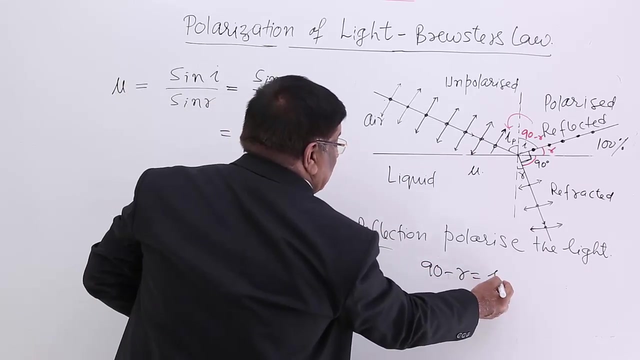 minus r upon sin r. What is this, cos r? Cos r upon sin r is equal to cot. I want to convert it into terms of i, not in the terms of r. So what is r equal? to answer: r is equal to 90 minus i, because we have proved 90 minus r is equal to i. So put this r on. 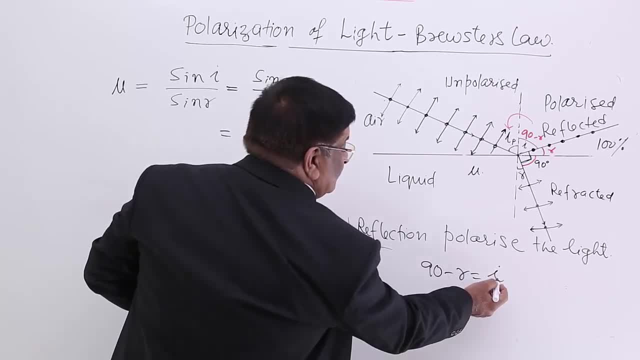 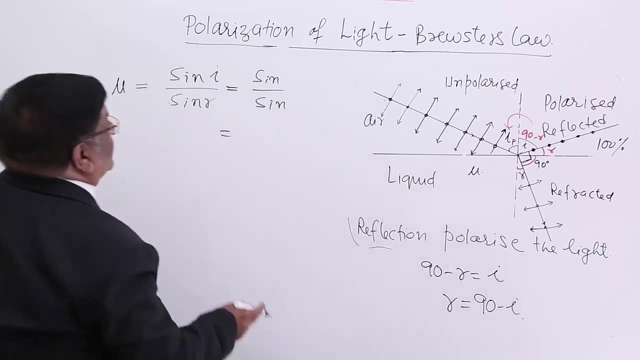 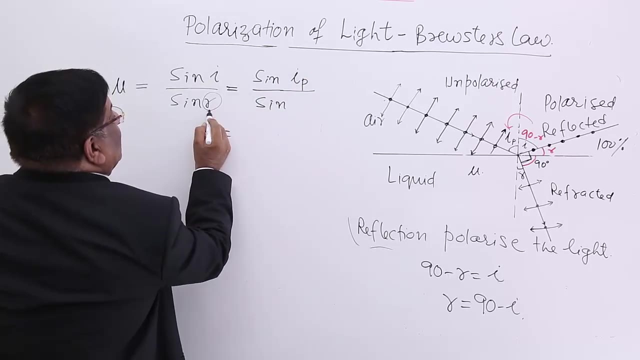 this side, i on this side. So how much r is equal to r is equal to 90 minus i. So I put it here: sin i is sin ip divided by r, and this r is equal to 90 minus r. and now it will be. 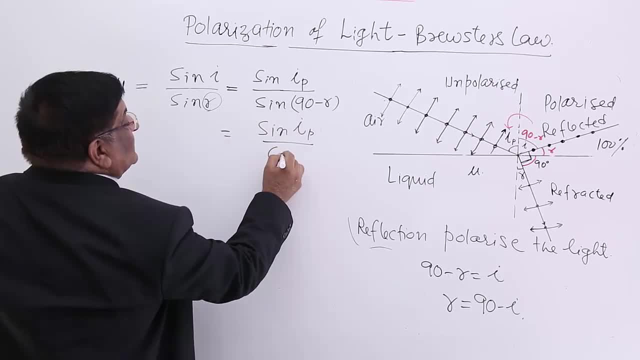 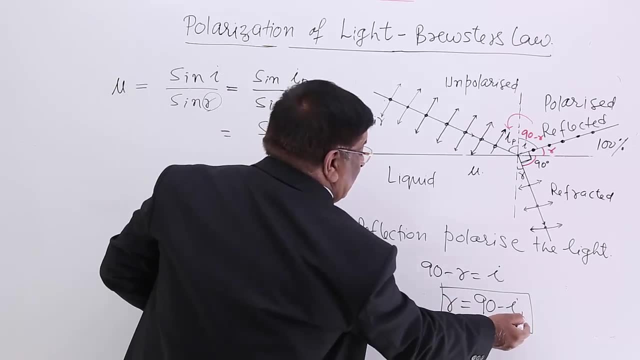 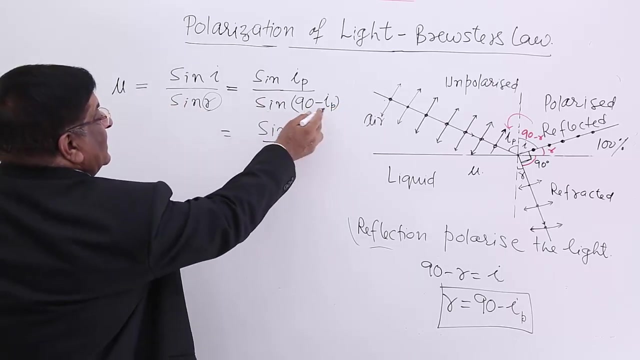 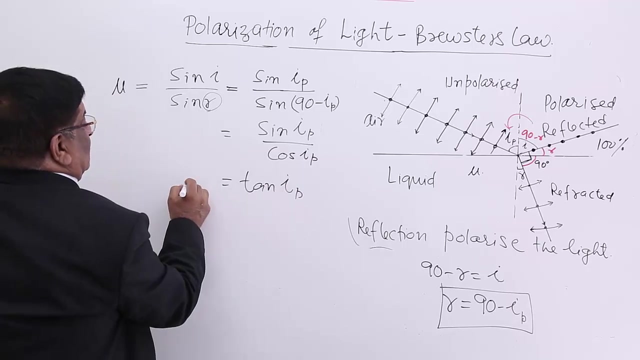 sin ip upon cos i r is equal to 90 minus ip. So 90 minus ip. now this is equal to sin ip upon cos ip. So this is equal to tangent ip. this is what mu, So refractive index of the liquid, is equal. 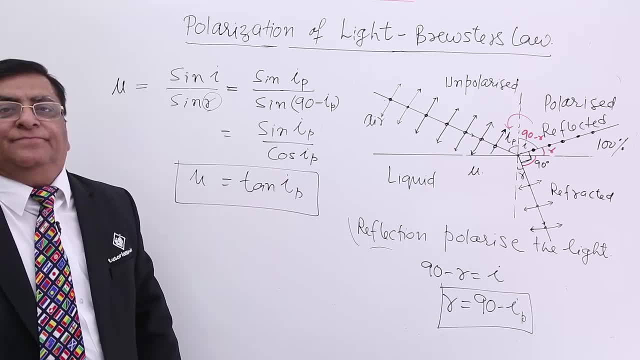 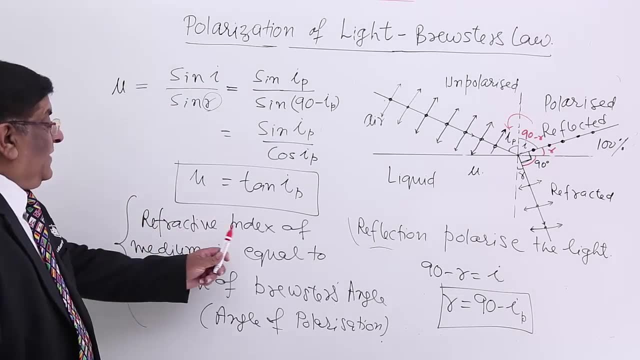 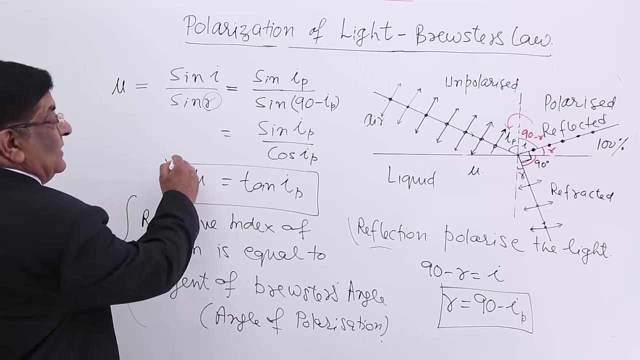 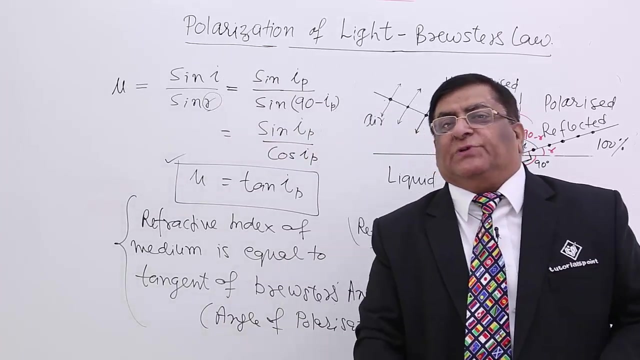 to tangent of the Brewster's angle. Again, Refractive index of a medium is equal to tangent of Brewster's angle, angle of polarization, and here is the small proof of this. So sometimes it is asked to us: what is Brewster's law? 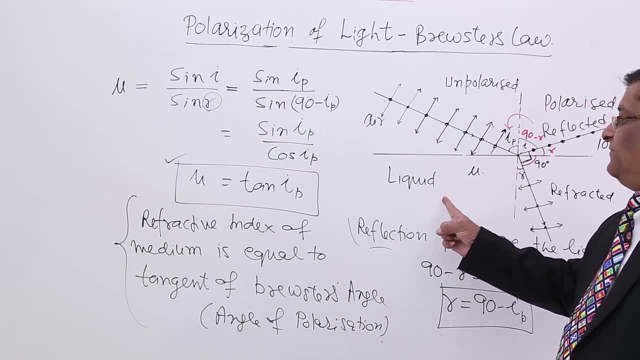 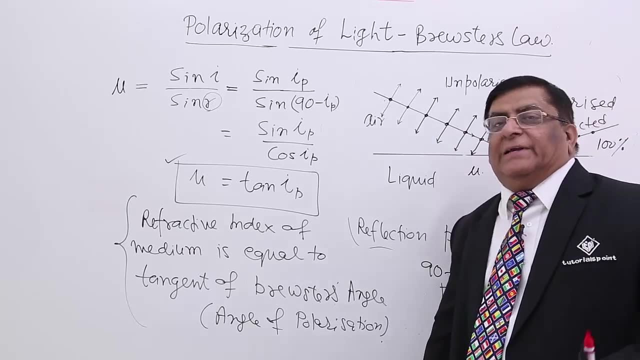 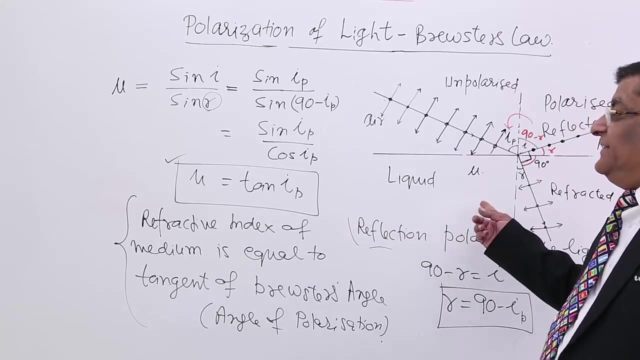 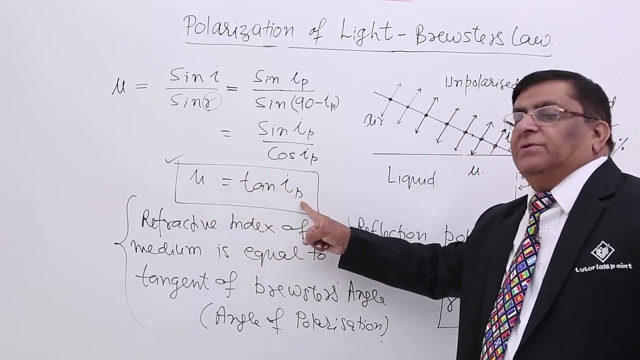 The Brewster's law is that refractive index of the medium is equal to tangent of the tangent of the Brewster's angle. So with this we can find out: if mu is given to us, we can always find out ip. and if ip is given to us, if ip we could find in practice, then 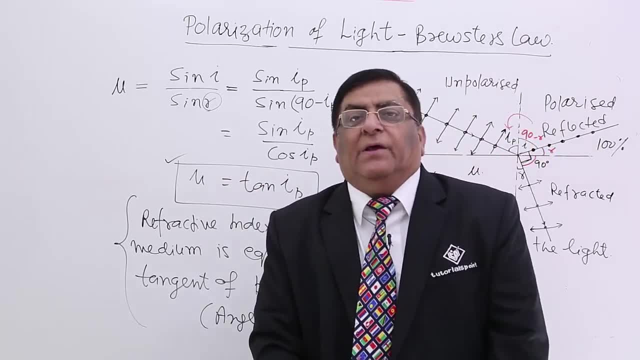 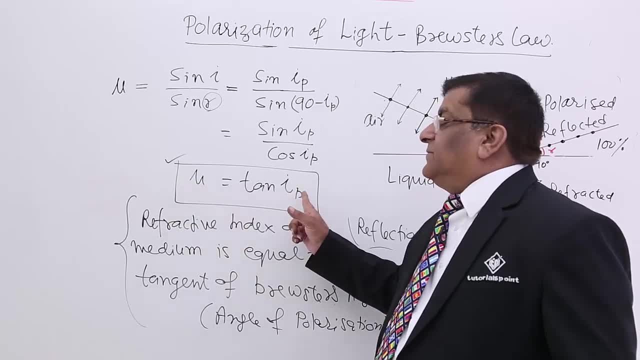 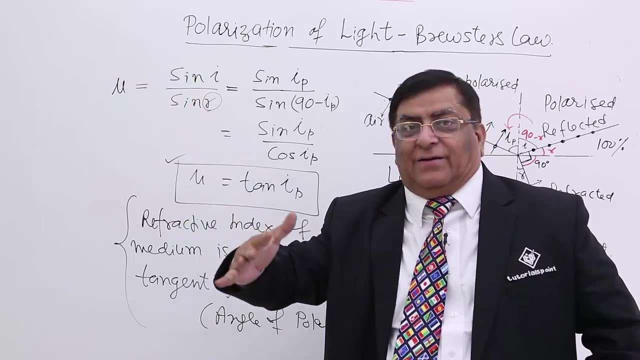 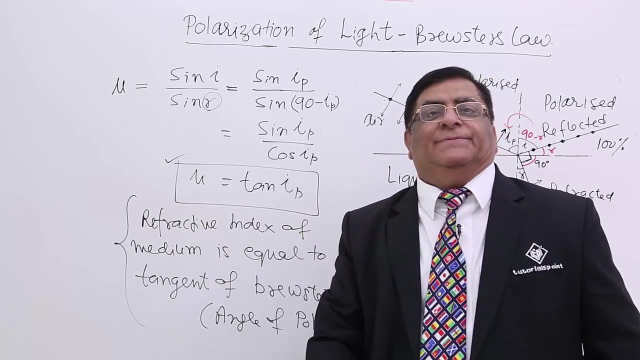 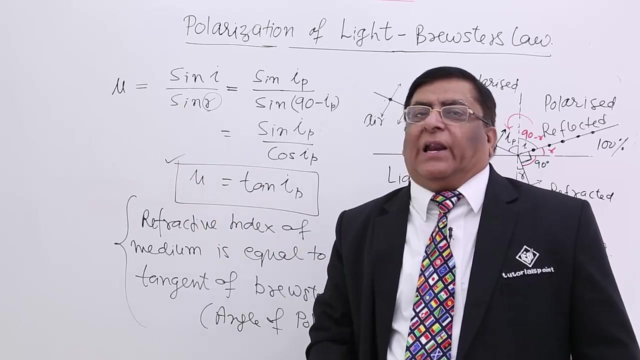 teeth. If the rays on the water at that angle are incident, then after reflection the light which is coming to us is totally polarized. So this is how we can find the light when it is reflected by water, The light when it is reflected by glass or by any surface. 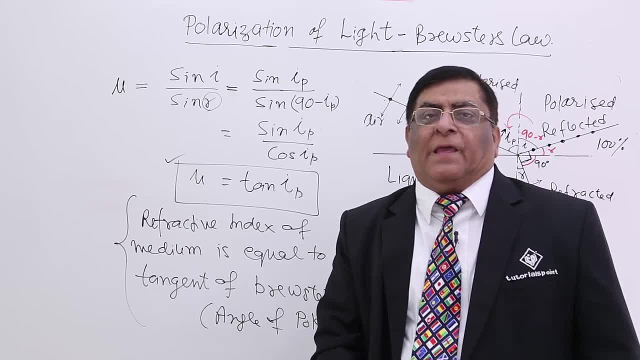 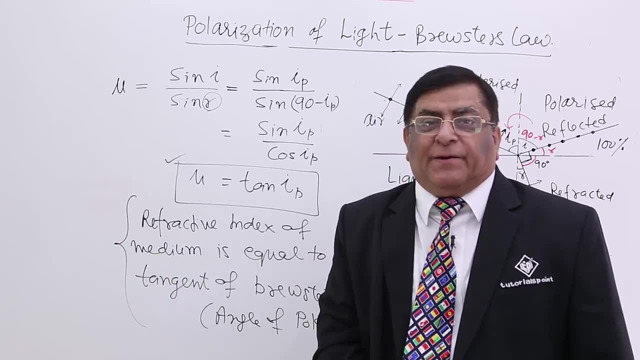 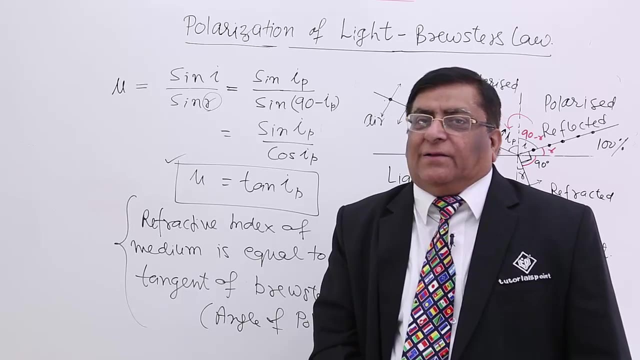 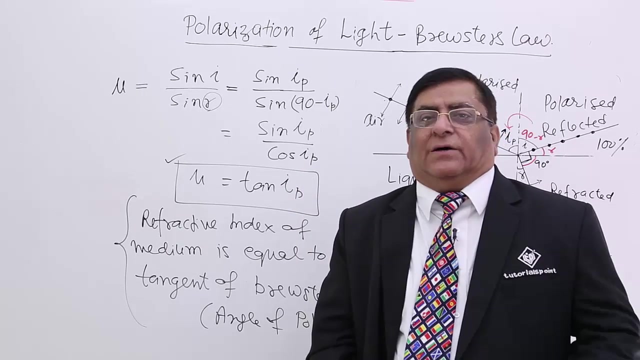 l other transparent medium. If we have to find out the light reflected by the road, we have to do the experiment, and that we can always do by using analyzers. We can find out at what angle the light gets totally polarized. So this is Brewster's law. and now in the next, 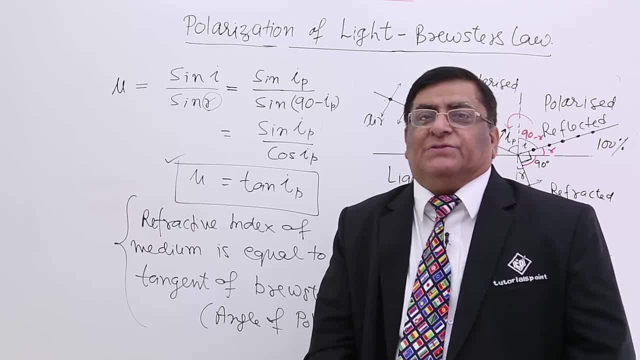 lecture we will see what are the applications of polarization. how do we use it? Thank you.